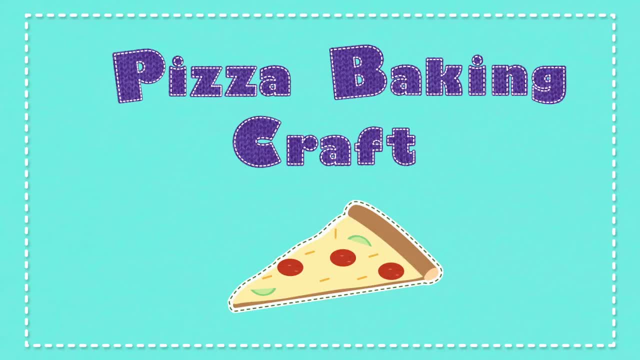 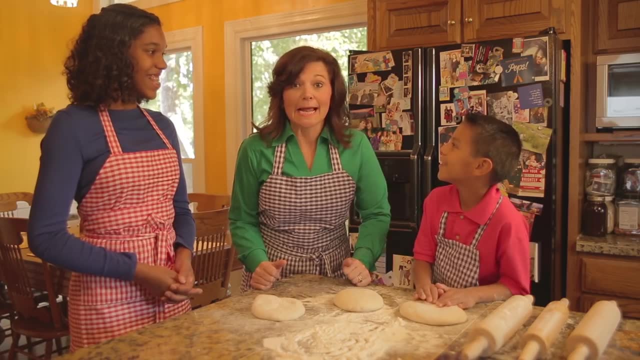 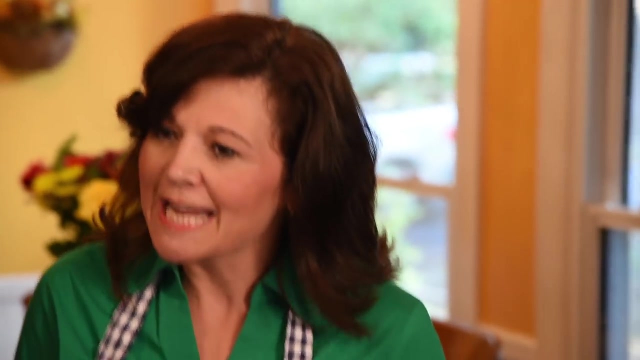 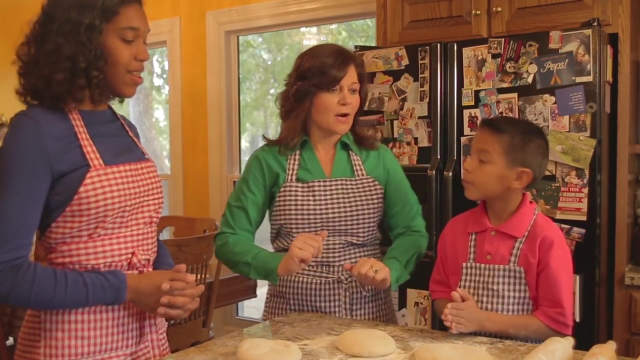 Pizza Baking Craft. Oh, hi everybody. I am Janet, and today we are in the Mother Goose Club Playhouse Kitchen and I am joined by my friends Anna Grace- Hello- And my friend Lucas, Hi. Today we are making pizza. We made our dough and now it is time to roll out our crust. Now, what we want to do is: 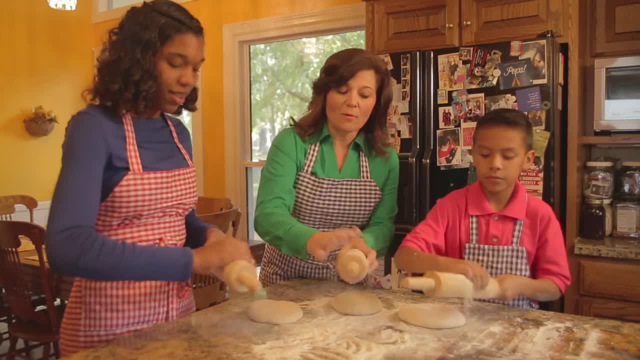 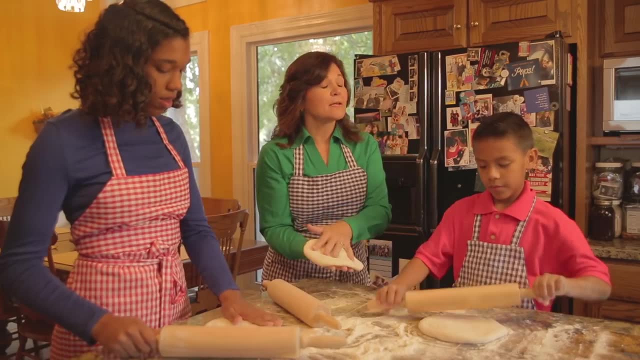 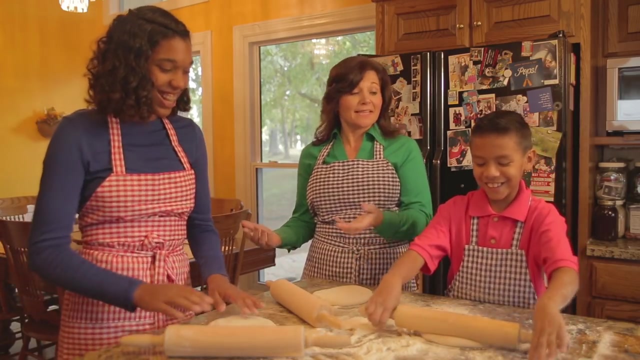 we're going to put a little bit of flour on our rolling pin. that way the dough won't stick to it so much. Let's get to rolling here. Here is a trivia question. Does anybody know who invented pizza? Gooey Lou, Gooey Louie- I love that name. I don't think he has anything to do with pizza. 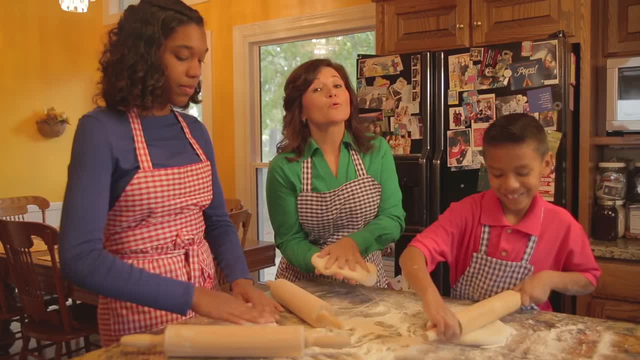 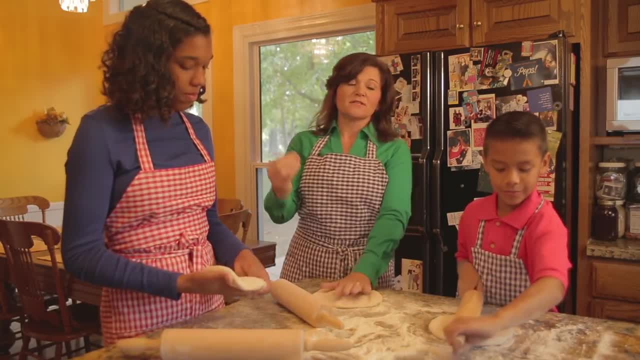 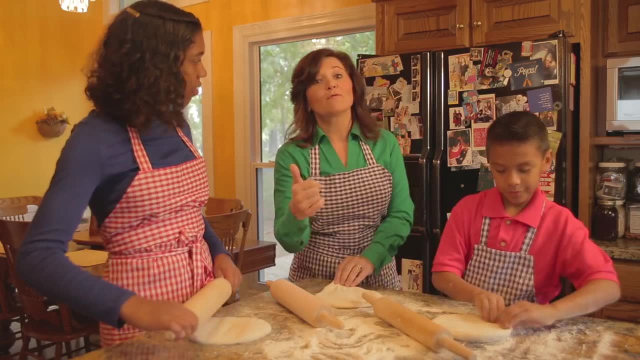 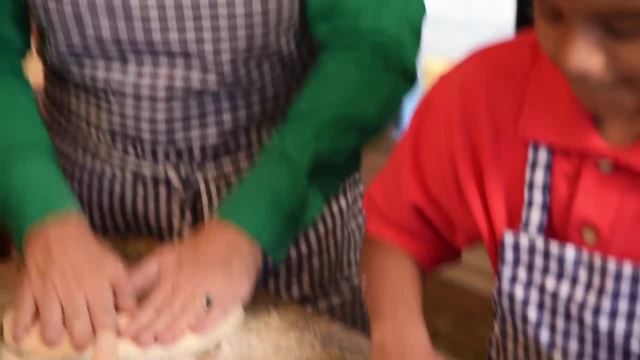 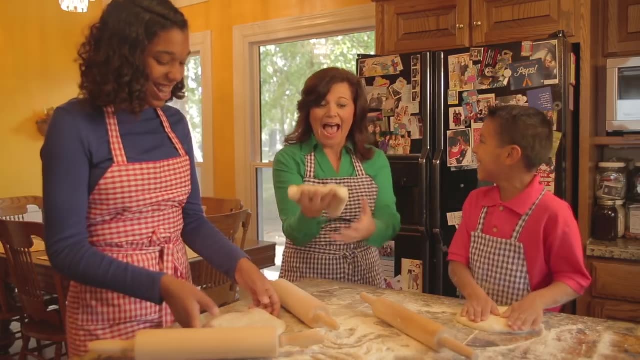 give Rafael Esposito some credit today for making pizza. All right, So I think that I'm good. Oh, I love it. You guys give it a try. That's kind of fun. It's kind of like action, like a frisbee. 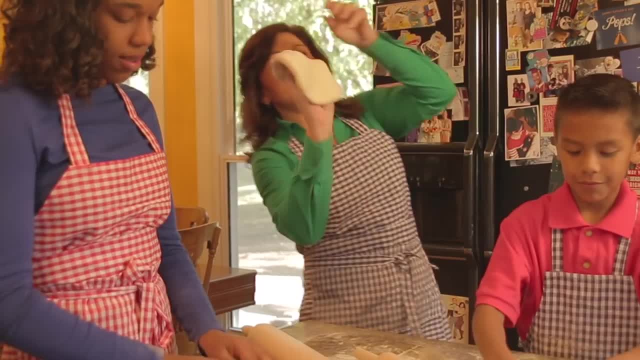 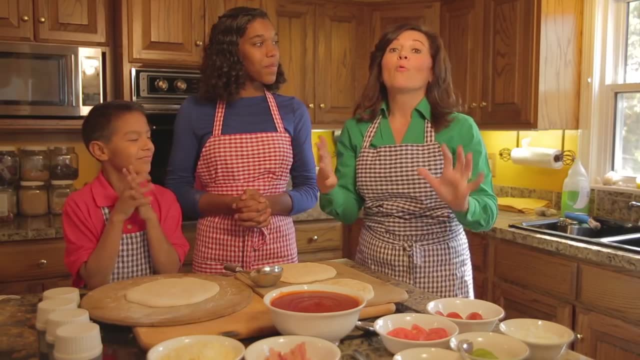 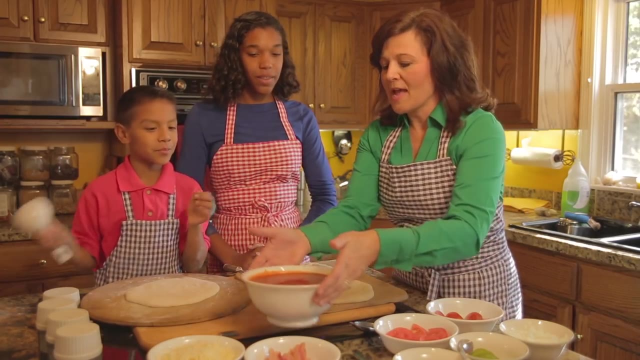 Yeah, Wow, That's good stuff. Oh yeah, One last twirl. So we have made our pizza crust. They're all looking very, very delicious. Now, what do you suppose is the first thing we need to do? We need to put pizza sauce on, All right? So, with that said, everybody grab a spoon and 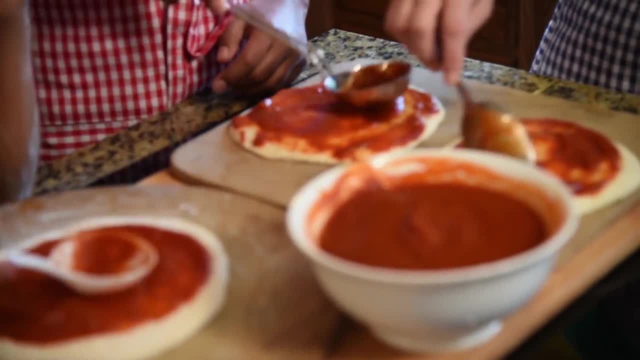 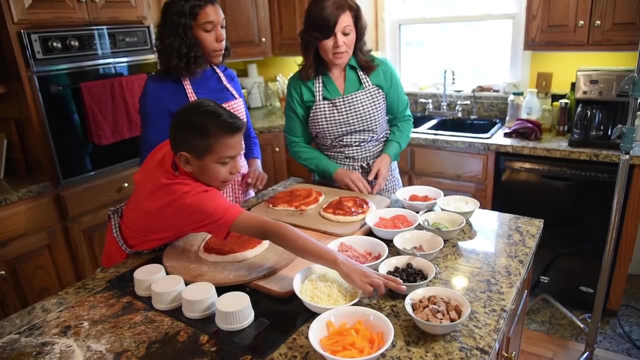 pizza sauce away, All right. So once you're fine with how much sauce you have on there, Perfect, All right. You guys are good with that, All right. Now we're going to talk about the ingredients we can put on top of our pizza. Now, you mentioned that you like what on your pizza. 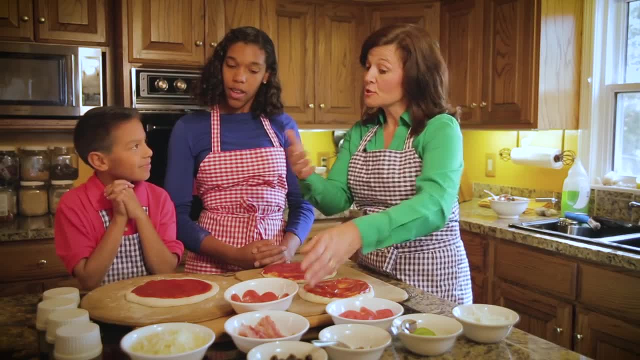 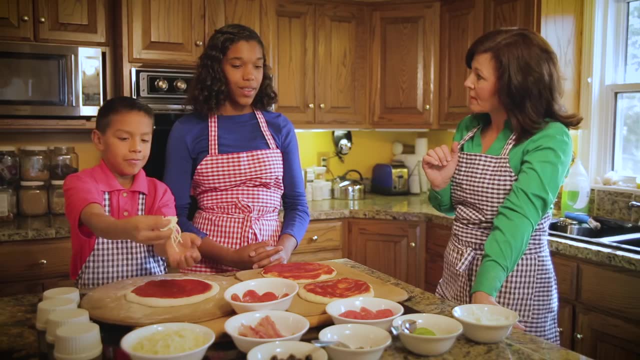 Pepperoni and cheese, All right. So are you going to put your cheese on first or your pepperoni Cheese? All right, So away you go. Now, what would you like to put first on your pizza? You know, I think I'm going to do something really funky: I'm going to put my cheese on last. 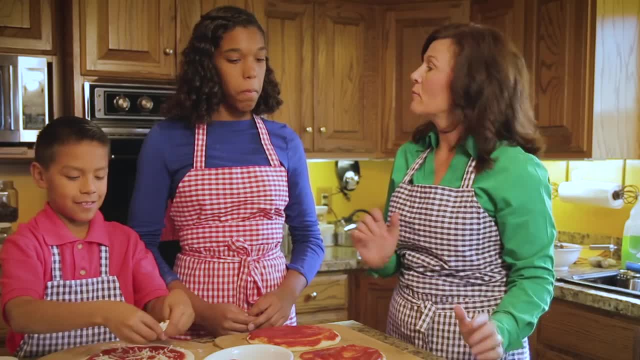 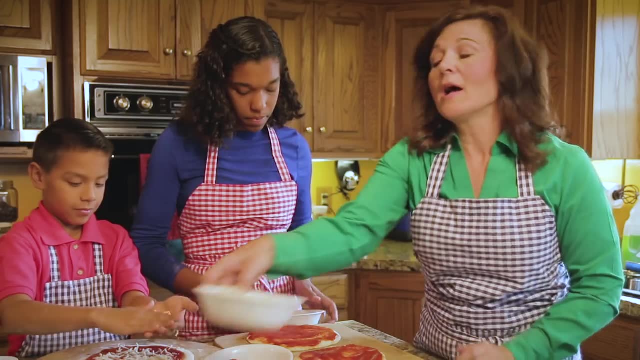 Ah, very, very creative here, All right. So what would you like to go with first? Probably bacon, All right. So she's going to put a bit of bacon Now. I am going to go the route of Chef Lucas over here: Put a little cheese. 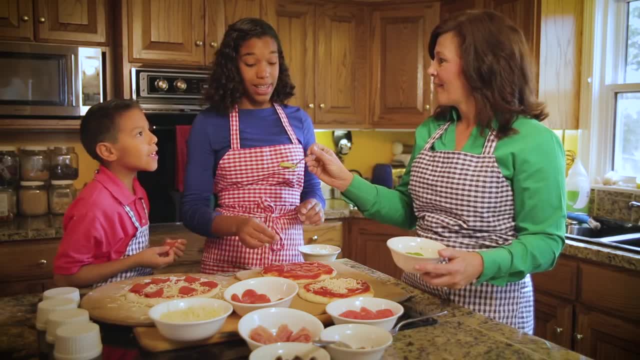 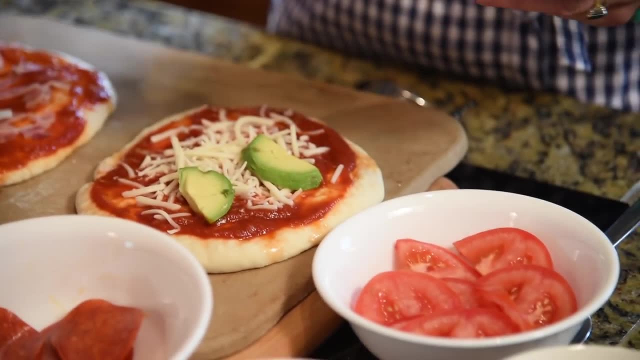 Have you guys ever had avocado on a pizza? Not on a pizza. Is that what you make guacamole out of? It is what you make guacamole out of, but I love avocado, So I'm going to put a little avocado here. 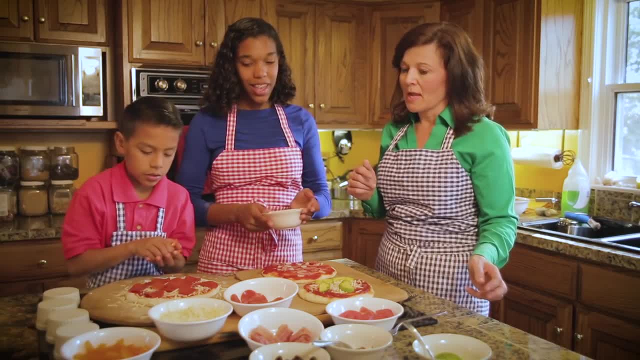 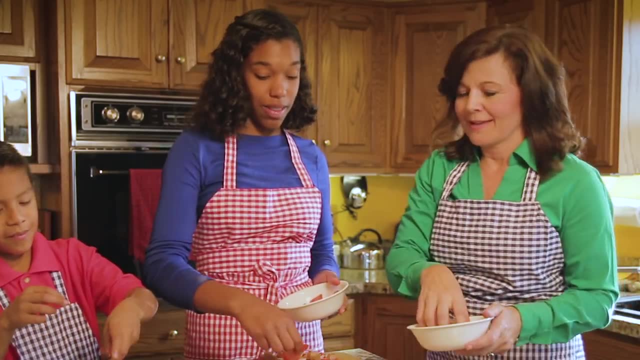 You're going to go for a little pepper there, A little orange bell pepper. I think that's a good idea. Now, where are you going to go from here? Sausage, All right. Oh my goodness. All of this smells so good. I just want to like eat it. 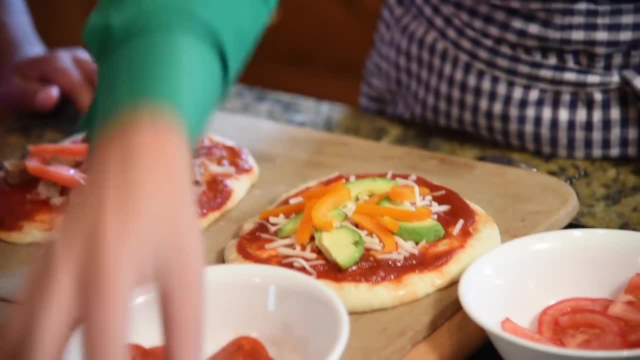 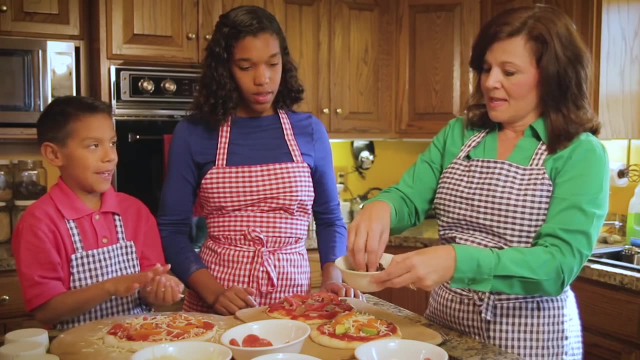 Oh, it won't be long now. And so I've got my peppers, I've got my avocado. I might go with a little more cheese, I might- Oh, you know what I forgot. That looks really yummy, And then I'm. 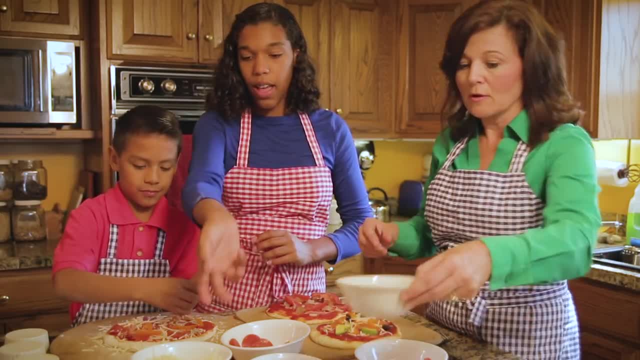 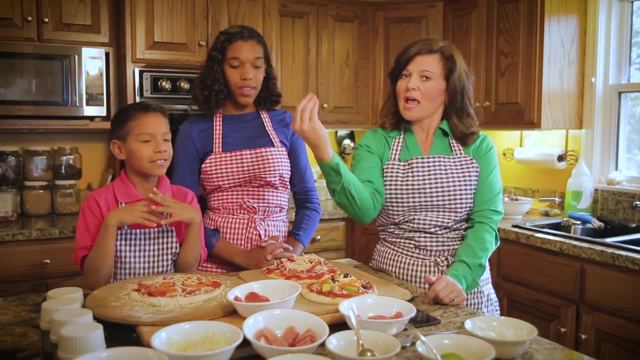 going to put some black olives on there just for good measure. There we go, All right, So now it is time to put the pizzas in the oven. Can you say la pizza? La pizza In the oven, In the oven. 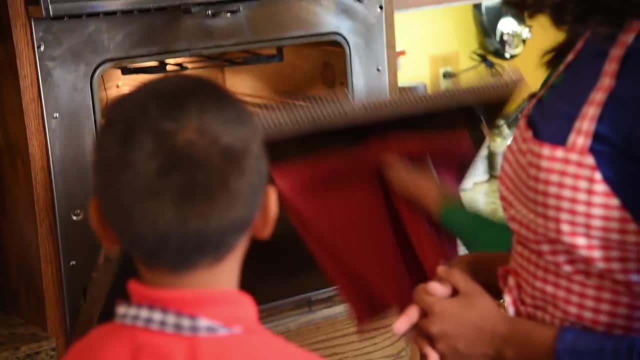 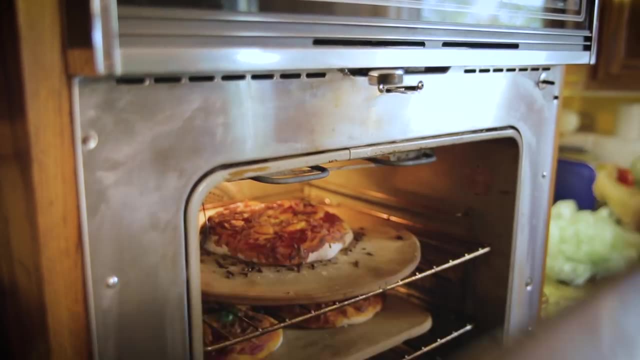 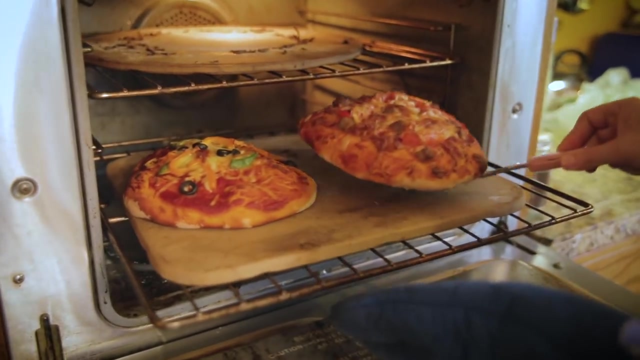 You always want to be careful with the oven and have some assistance with that, And now we will set our timer, All right, And we wait. Oh goodness, This is Lucas's pizza. We're going to put that right there. This is Anna Grace's pizza. 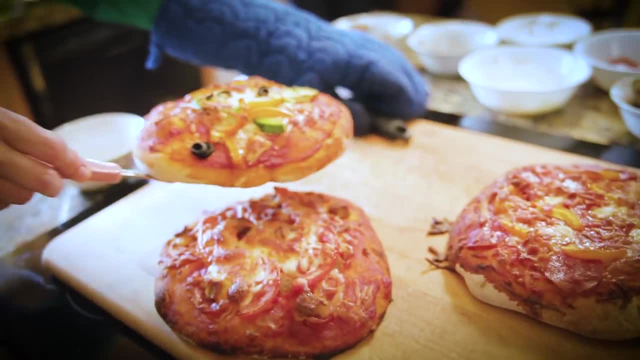 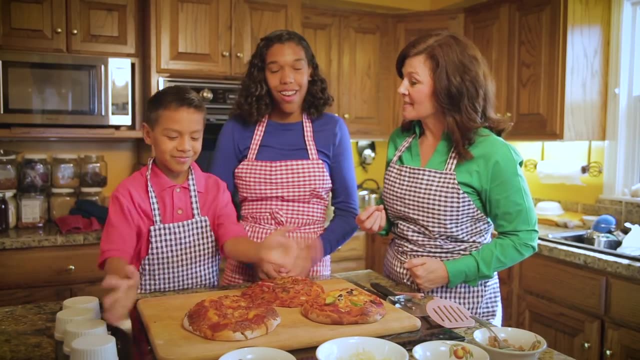 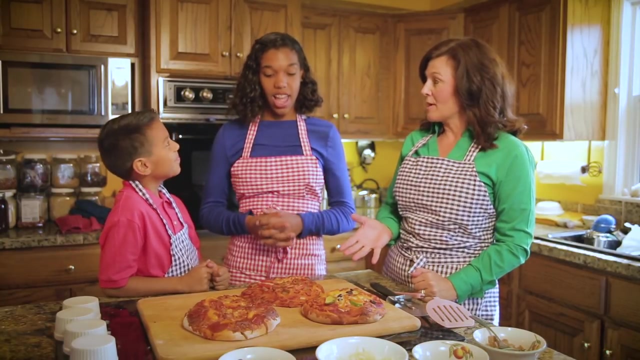 And then this is my pizza. Do these not look amazing And they smell fantastic, don't they? Yes, Are you proud of your creation? I think it's going to be really good. All right, And you're excited to try yours. I say it's time to cut into these pizzas and let's have a bite. I think the